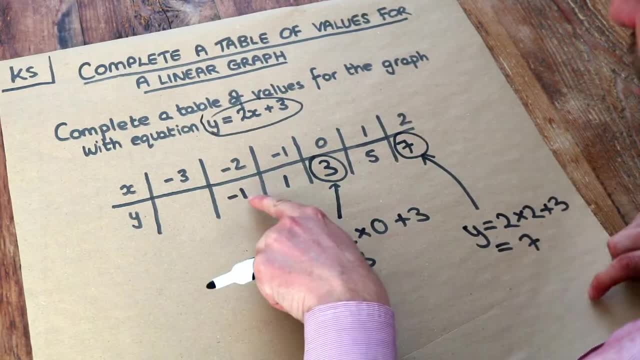 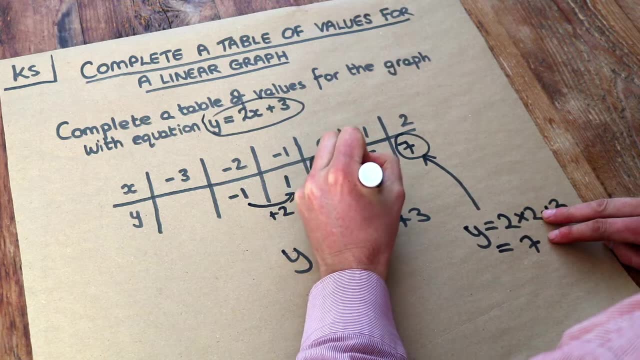 Now you might have spotted a pattern by this point. Can you see the y values are going up by 2 each time. Look, plus 2,, plus 2,, plus 2,, etc. And in general, whatever it's going up by will be the number in front of the x. 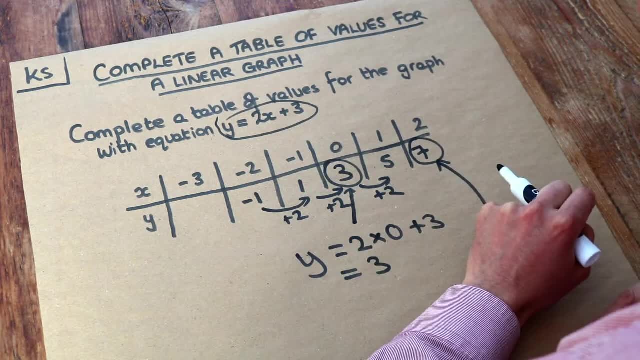 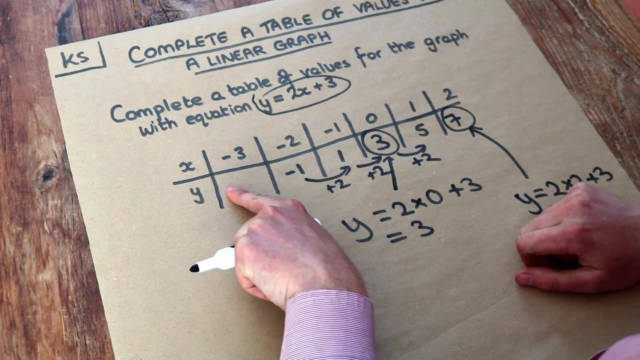 So if it's 2x, then these numbers are going to go up by 2.. So we could therefore work out what this value is without having to substitute minus 3 into this. Well, if we go down by 2, we can see it's minus 3.. 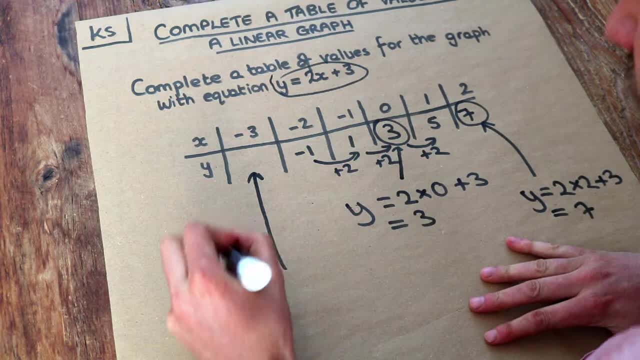 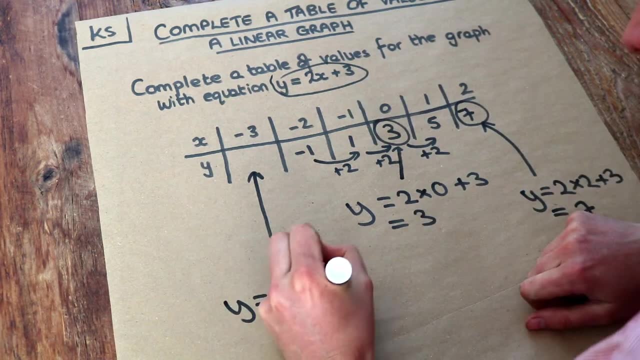 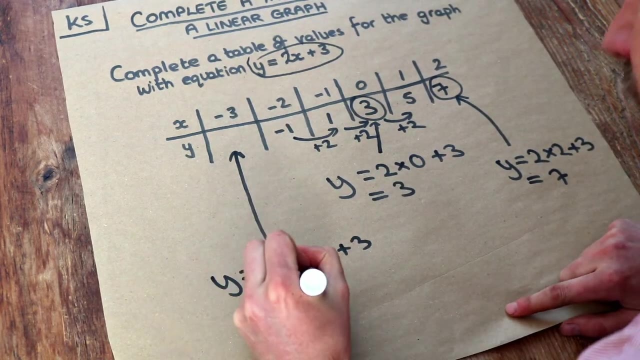 But let's just work it out in the same way as we did before. If the x value is minus 3, y is 2 times minus 3, 2x, 2 times minus 3, plus 3.. Now, 2 times minus 3, positive times negative is negative, so it's minus 6, plus 3.. 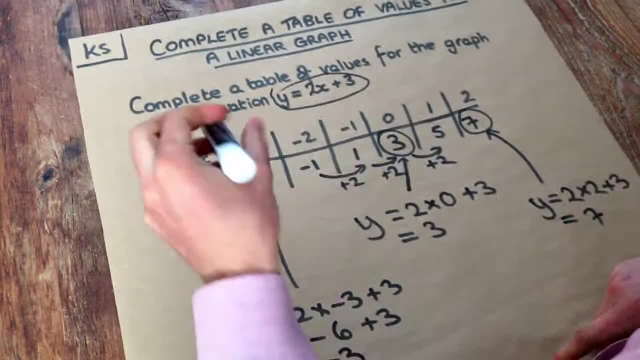 And what's minus 6 plus 3?? It's minus 3.. So, indeed, we get the value we expected, which is minus 3.. 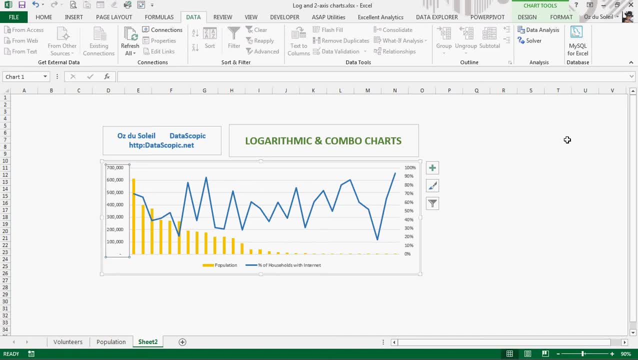 Hello Oz Dusilay here with Datascopic and I'm going to show you about making a meaningful data representation using the logarithmic axis and making a combo chart. But so we're looking here at city populations and percent of households that have Internet connections. 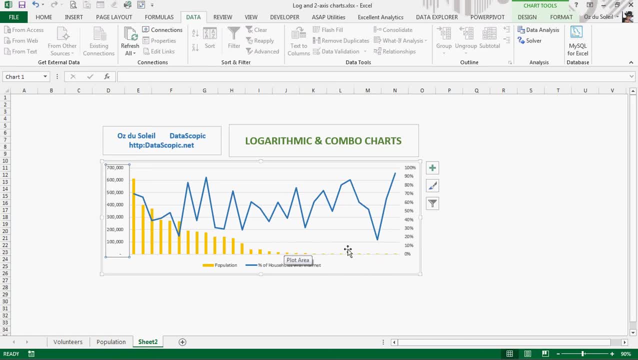 And we have these really small numbers that are hard to analyze. We don't know what's going on there. We know that they are somewhere under one hundred thousand, but we don't know what they are. And then we have this at six hundred and fourteen thousand.